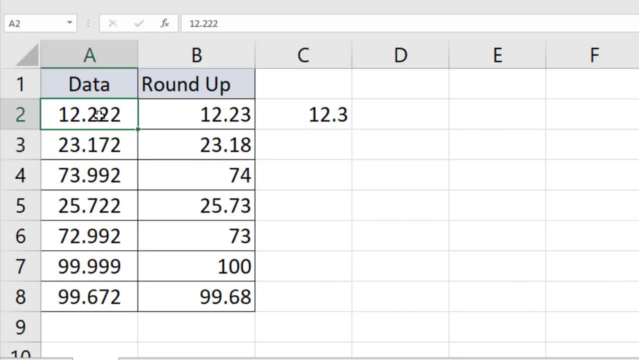 close parentheses. press enter. See 12.222 could be round up at 12.23 and it could be round up to 12.3. only This is how you can use roundup function in Microsoft Excel, Thank you. Thanks for watching. See you in the next video. 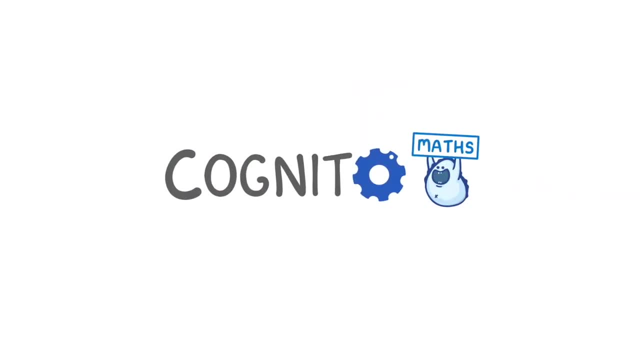 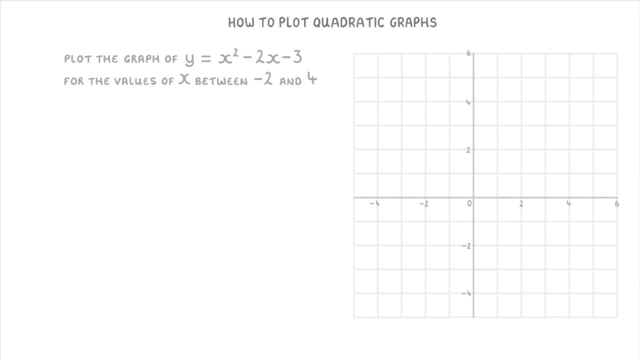 In this video we're going to cover how to plot quadratic graphs. For example, in this question here we're being asked to plot the graph of y equals x squared minus 2x minus 3.. And we only have to plot it in this region between where x is minus 2 and where x is. 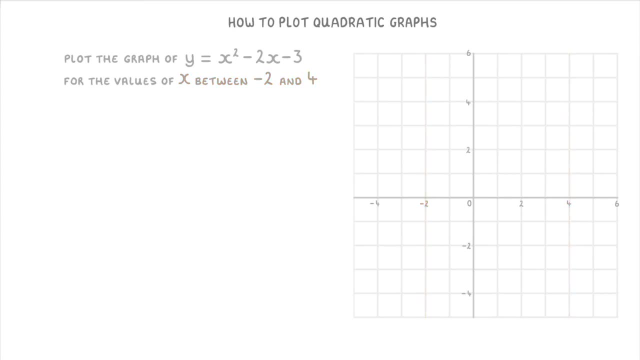 4. Whenever you're asked to plot a graph, you're basically being asked to work out a bunch of points that the curve will pass through, and then join them all up with the curve. To figure out where the points are, though, it helps to use a table like this. 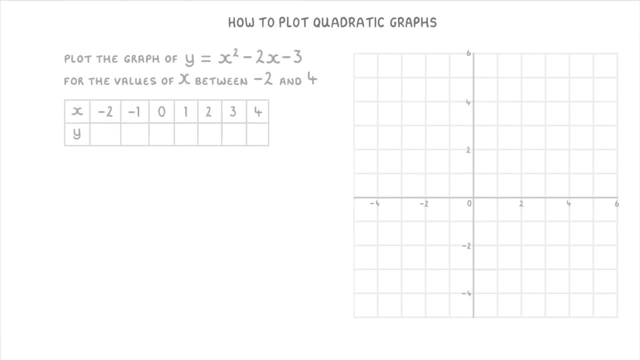 On the top row are all of the x values within the range that we're trying to plot, So in this case all the whole numbers between minus 2 and positive 4.. Then on the bottom row we can add all of the corresponding y values, For example: 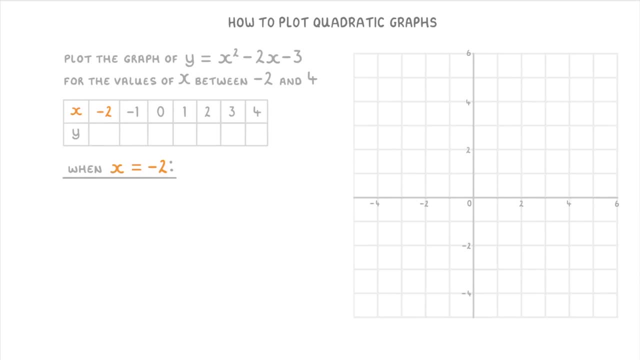 when x equals minus 2, we can figure out what y will be by plugging minus 2 into this equation that we were given in the question. So y will be equal to minus 2, squared minus 2 times minus 2, minus 3.. Which simplifies to 4 plus 4 minus 3.. Which is: